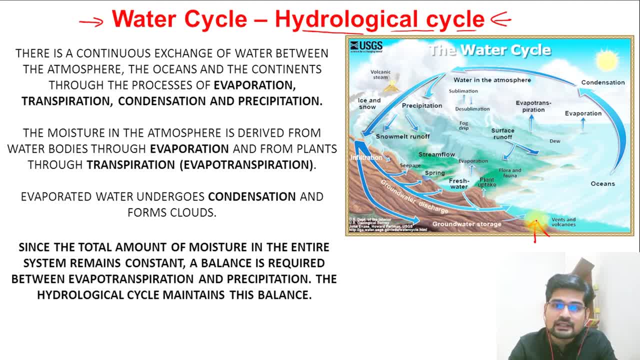 is the global climate. So hydrological cycle is one thing that we need to understand, and also the factors related to it, And later on in this session we are also going to talk about various forms of condensation and their characteristics. So hydrological cycle, 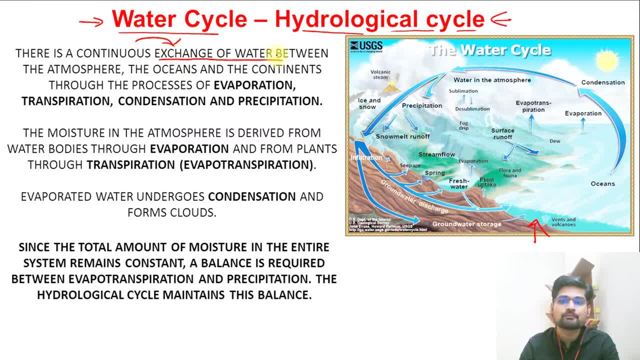 as you know, it is a continuous exchange of water. Now, this exchange of water, do you see here what happens? in the earlier lectures Also, we have talked about the exchange of water between the oceans and continents. We also talked about various kinds of circulation of air and water. right, 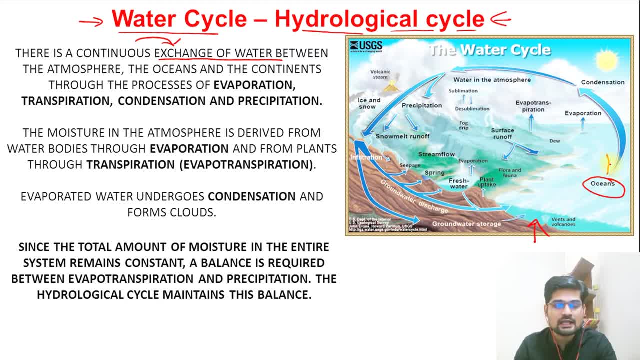 So moisture becomes very much important. So what happens at the ocean of the land water? It evaporates right and then it goes up, and where the cloud formation happens, And when it reaches a dew point, remember- then saturation happens and then rainfall happens. So we have already. 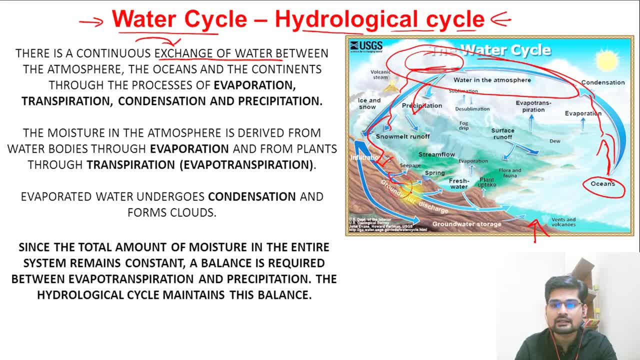 understood this, and again this water is coming back to the land, and again it flows through the rivers to this particular oceans. So this is a complete cycle that happening and in this cycle there are few processes that are very much important. so at first step that we understand is the process called. 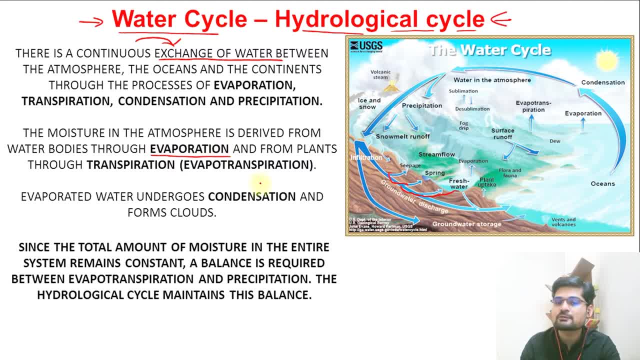 evaporation, right then what we have is the process of condensation. so first is the evaporation process, then evaporation happens, and further in the atmosphere- remember what happens- condensation starts. so during this condensation, again, there is a heat change, which is called latent heat, which is released. right so 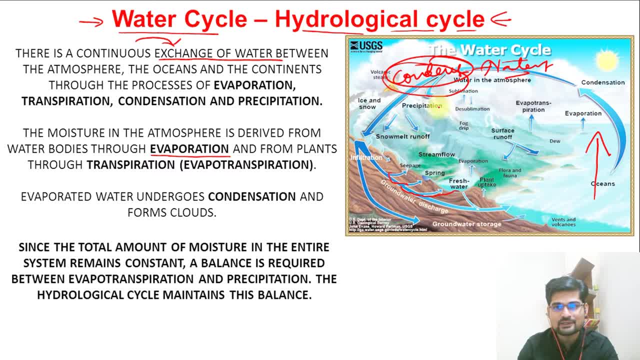 this is also important, which we have learned in the concept of tropical cyclones as well. right and apart from this, there is something called transpiration, remember that happens from the green leaf of the plants, through these pores. that is what water is released. so this is called transpiration. 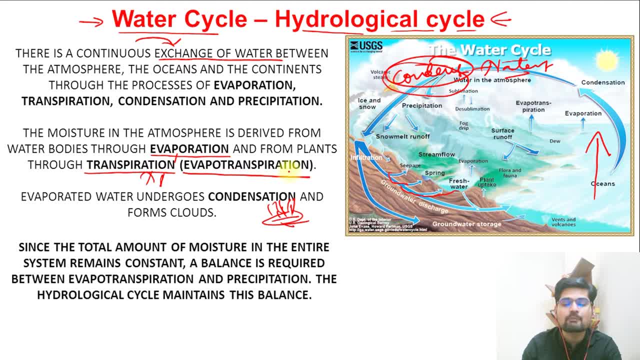 so evaporation and transpiration together they are called a vapor transpiration, and that is important to understand. so this is what is related to the concept of the circulation of water right. so evaporated water under goes, then condensation and they form clouds, and then again what happens? 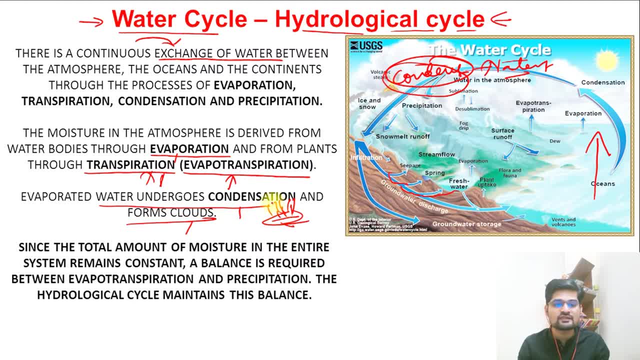 through the clouds, if rainfall happens, the water again comes back to the surface. so, since total amount of moisture in the entire system remains constant, now here is the catch: in this entire cycle, what is constant? the total amount of moisture, right, so this is important to understand. the same amount. 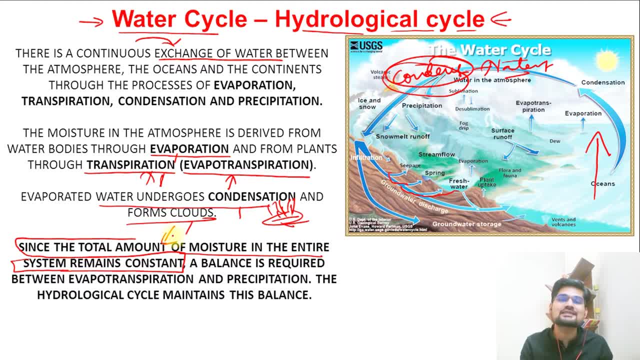 of moisture is there in the entire system, which is kept on circulating and circulating. so that is important to understand. now why are we studying it? to understand how it is balancing the entire system. so a balance is required between evapotranspiration and precipitation. so remember evaporation and 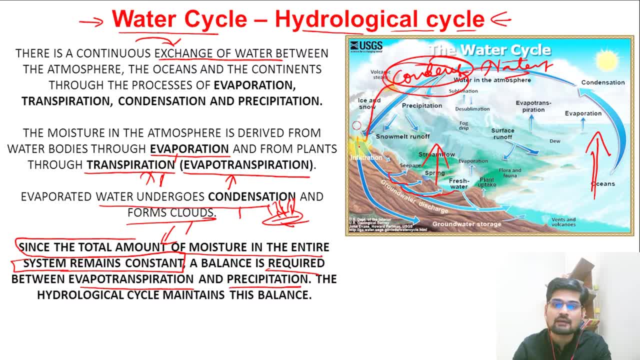 transpiration happening and then the condensation happening. so it means this is something like input and then output. so input and output has to be in a balance that we talk about. so this is that balance which is maintained by which cycle? hydrological cycle, this balance between evapotranspiration and 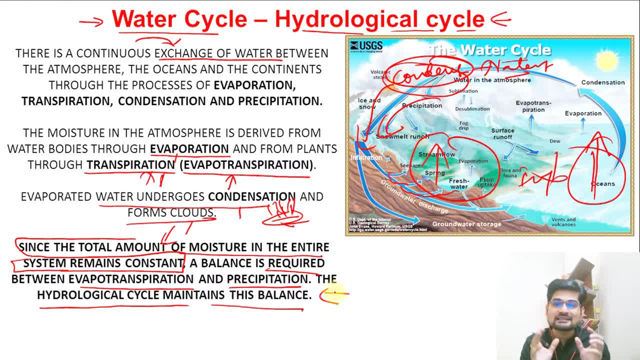 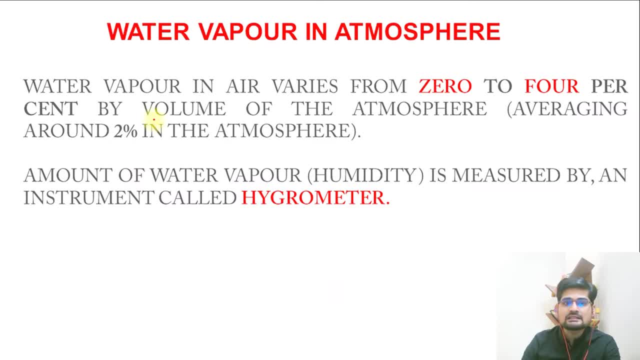 precipitation or condensation that we say. it is this particular balance which is important for the climatology. now let's elaborate further more. now let's understand this content, that is, water vapor in atmosphere. so water vapor in air varies from 0 to 4 percent by volume. now, remember, this is 0 to 4. this range is 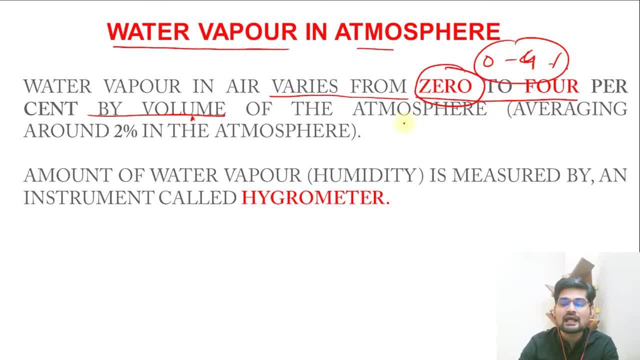 important maximum. it is 4 percent by volume of the atmosphere, if you see so averaging around how much 2 percent in the atmosphere. so maximum is up to 4 percent. that is important. so amount of water vapor, that is, humidity, is measured by an instrument which is called hygrometer. and remember we have already discussed 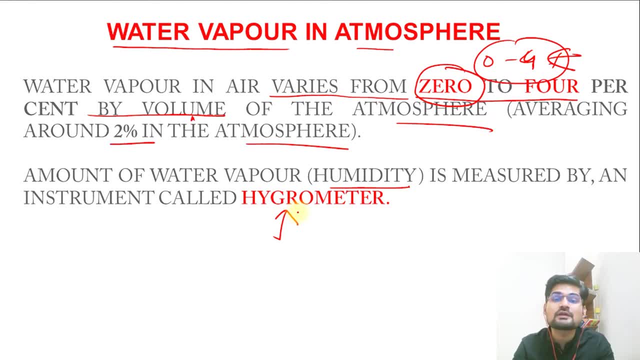 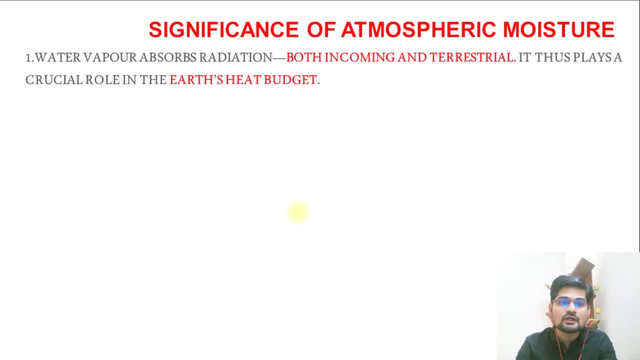 in the humidity, the various kinds of humidity. so that is where water vapor is measured in per unit volume of air. so it's important. so significance of atmospheric moisture is what we need to learn. so first important point is that water vapor absorbs radiation, both incoming and terrestrial. remember that. 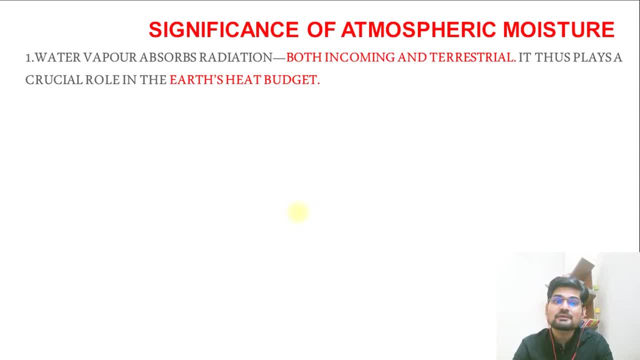 is important in heat, which it also. we discussed about this. so water vapor actually absorbs radiation and it just plays important role in what in earth's heat budget maintenance. then what we have is the amount of water vapor present decides the quantity of latent heat that will be. 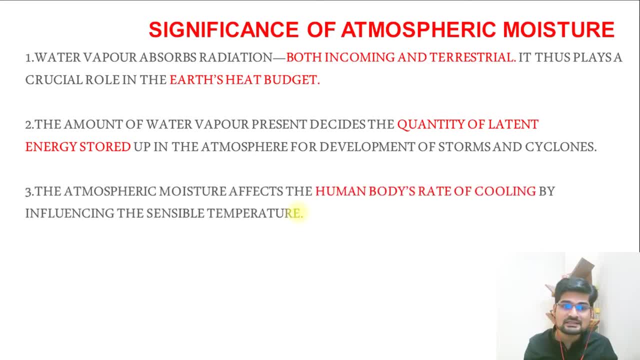 stored, remember. so that is important here. then what is here? the atmospheric moisture affects the human body rate of cooling as well. so that is where it is concerned directly with human beings, right? so human body is rate of cooling by influencing the sensible temperature that we say, right, the room temperature. 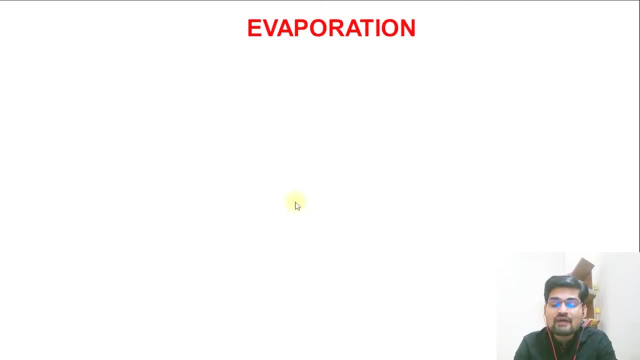 temperature, remember. so that is also important. then evaporation is another factor that is important. so what happens here? let's see: oceans covering 71% of earth's surface hold 97% of the earth's water. that is important to understand that ocean. in terms of area, it has 71% of earth. 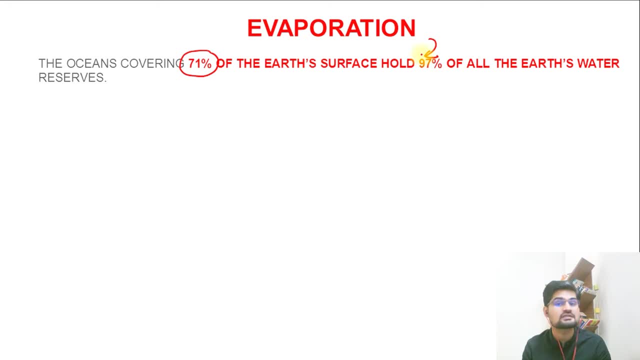 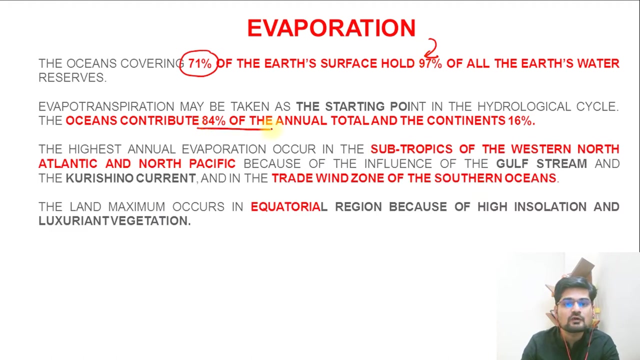 but it covers 97% of earth's water reserves. that is important. so maximum evaporation happens where? in the oceans only so evaporation may be taken as the starting point of hydrological cycle right, so that is important. and further, if we see the oceans contribute to 84% of annual total, 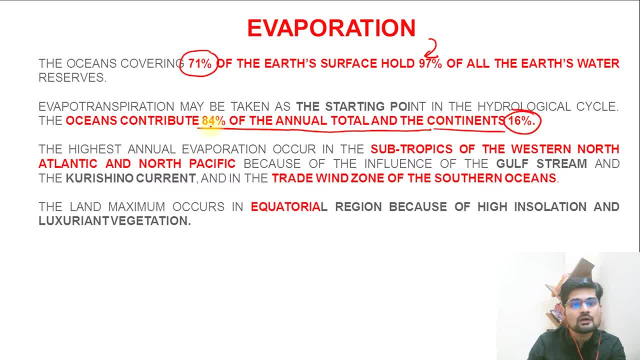 and the continents. that is 16%. so, remember, oceans are the maximum controller, or maximum contributor, in that way, to the hydrological cycle, while the land masses are contributing this 16%, remember that is one of the important key factors. so, distribution of land and water, 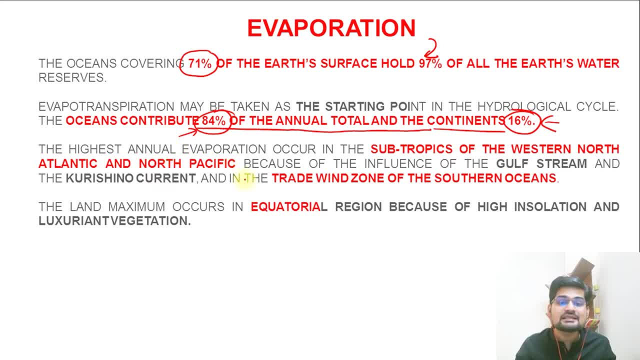 becomes one of the really important point now: highest annual evaporation. remember where it occurs: subtropics of Western North Atlantic and North Pacific. and why? because of the influence of these Gulf Stream, that is, warm ocean current and Curacao current, and in the trade wind zone of these southern oceans as well. so these are the regions where evaporation is. 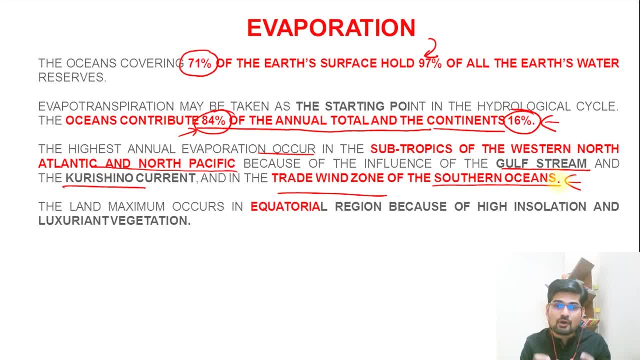 maximum. so remember maximum evaporation. subtropics to the trade wind belt, that is the maximum insulation belt, so you have maximum evaporation also occurring there, only land maximum. remember maximum evaporation on land, which is called land maximum, occurs where in equatorial region because of high insulation and luxuriant vegetation. so remember evaporation as. 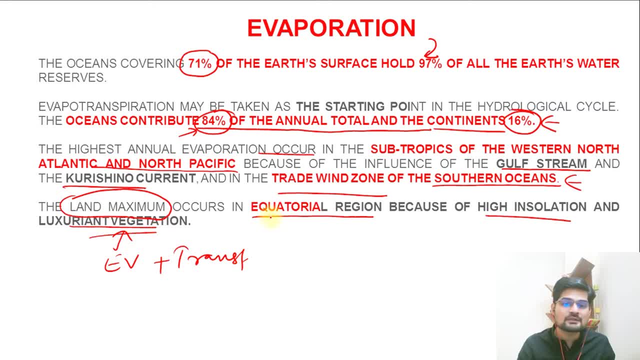 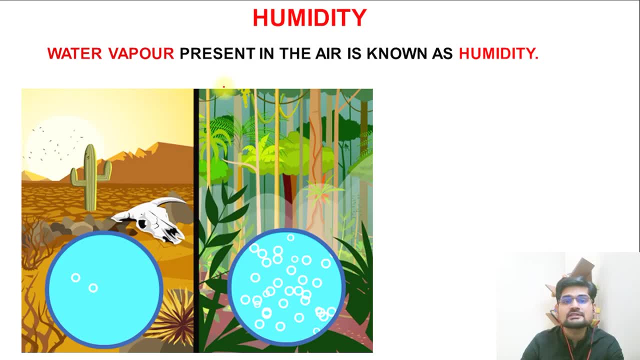 well as transpiration through the leaves. that is why it happens maximum in equatorial region, in the land areas specifically, if you see right. so that's important. now we have talked about certain components in the earlier lectures as well. for example humidity, which is important component of hydrological cycle. for example humidity, which is important component of hydrological cycle. but 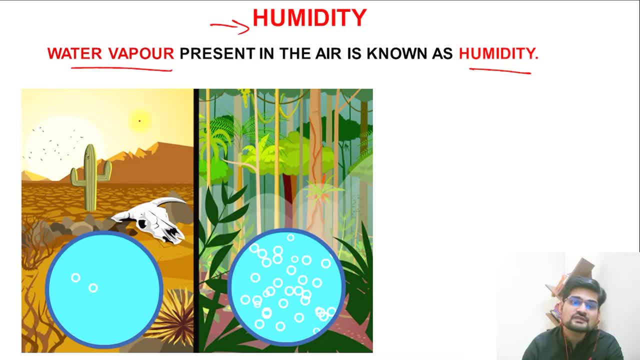 basically means water vapor present in the air, right? so if you see, this is a dry condition and this is a wet condition, so you have different situation here, right? this is important to understand in terms of humidity, so if you have not watched the video on humidity, please go there for. 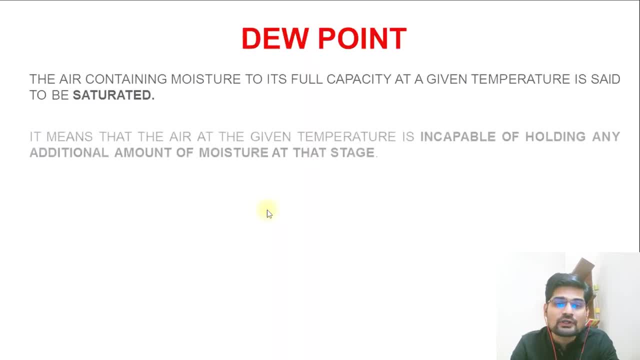 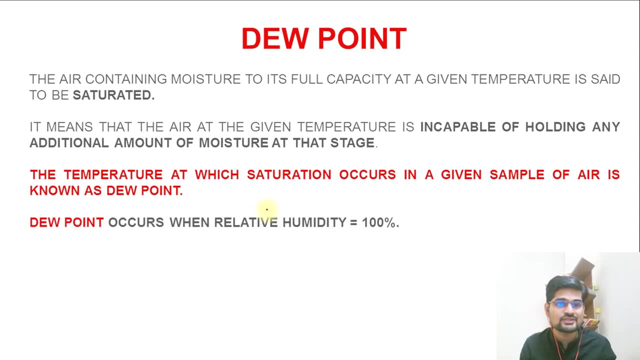 the details as well. then we also discussed about this dew point concept, right, so it is also important in terms that we need to understand what is dew point and its significance in climatology. so the air containing moisture to its full capacity, what is called saturated air, and that point that 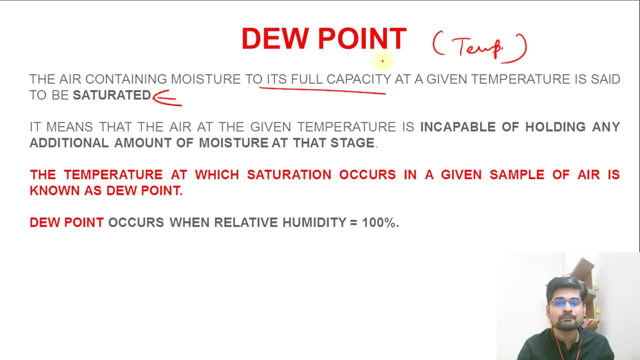 temperature. basically, if you see right, a particular temperature where this saturation occurs, that is called dew point and remember this is important for your cloud formation and rainfall or precipitation. right, because now the air is saturated, it cannot hold any more moisture, so any more moisture it means the rainfall will start happening. so dew point occurs where relative humidity is 100 percent. 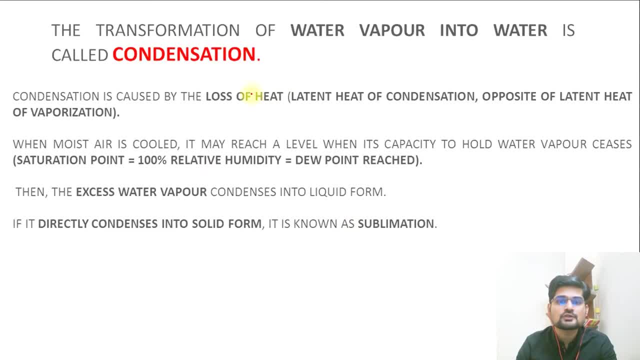 that we have discussed in detail in the previous lecture as well. so now we have already discussed about the evaporation of the air. so now we have already discussed about the evaporation of the air. so now we have discussed about the evaporation of the air. so now we have already discussed about the evaporation part, or transpiration part. 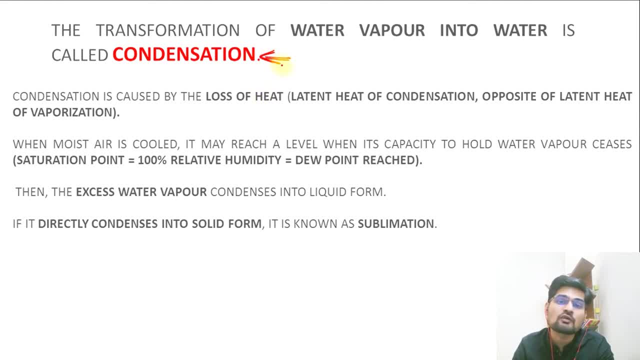 now let's understand the condensation: part of precipitation, part of the hydrological cycle, so transformation of water vapor into water. this is the basic definition of what you say is condensation. so condensation is caused by what? now here is the catch: loss of heat. remember during the 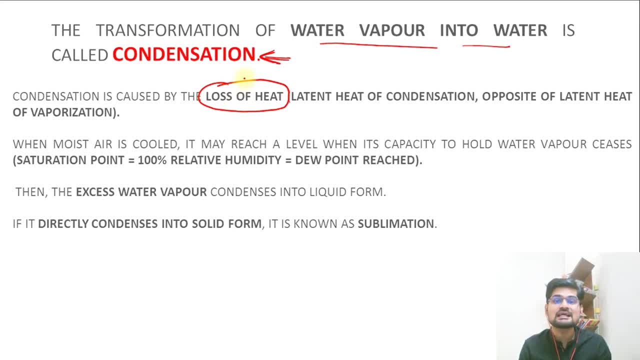 evaporation, heat was absorbed, right. so that was actually absorbed by the vapor. so that is also called vaporization or heat of vaporization, right. but here what you see during condensation: now it is cooling down and energy is actually released out by the system, and that is what we. 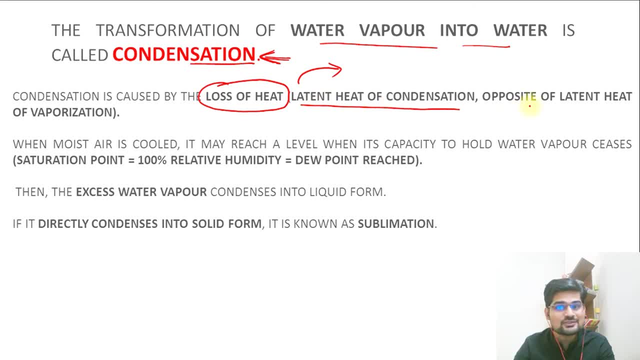 understood as latent heat of condensation. remember, just opposite, the latent heat of vaporization, which is absorbed, right. so that is important to understand. and when moist air is cooled, now remember, when there is a vapor and it is cooled, what happens? it reaches a level when its capacity 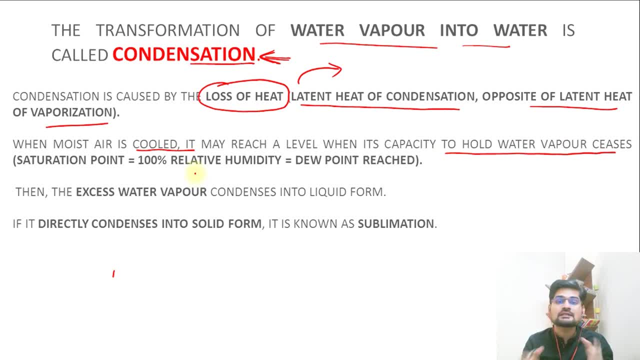 to hold water is actually done, so it's maximum. it means now it has reached hundred percent. so it's actually done, so it's maximum. it means now it has reached hundred percent. so saturation point is hundred percent. it means relative humidity is the hundred percent factor. now no more water can be stored, remember, in that particular air. so that is called. 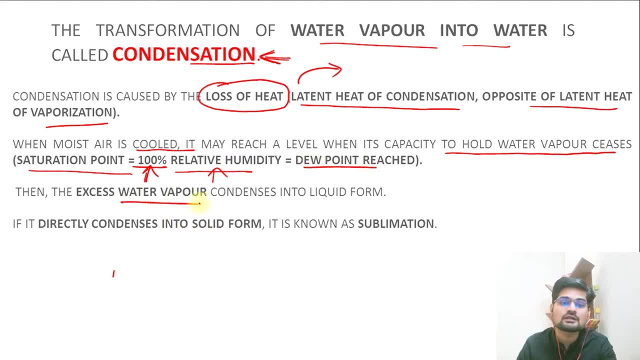 dew point, as we remember. so then this excess water condenses into liquid form, and this is that process. what we say is condensation happening, right. so if it is directly condensing into solid, remember now, if there is a vapor condition it goes into liquid- then it is condensation, right. but if directly it solidifies, then what it is? 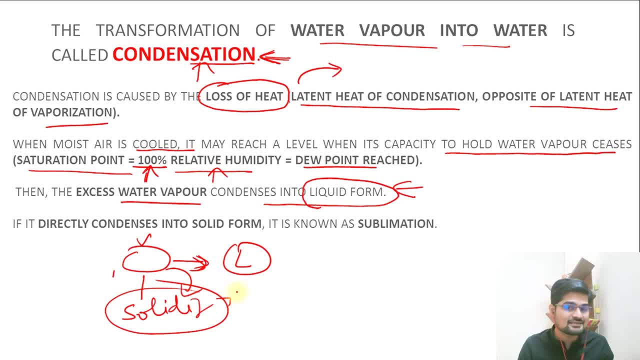 called. if it converts into directly into solid, that is, ice crystals, it is called sublimation. remember that is the difference between our condensation and sublimation. so many times what happens? this cooling starts happening abruptly, right? so in that case sublimation happens. that is where you see blizzards. 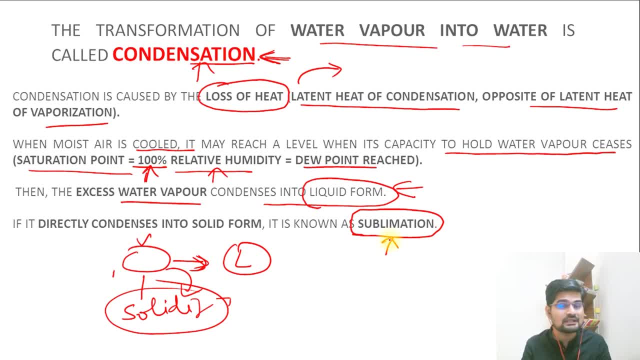 hailstorms- right, those are important- snowfall happening. so this is what we say is that condensation has two forms. if you see, one is gradual condensation and one is directly into solid forms, so it can be the precipitation of different forms that we need to understand. so now let's understand various kinds of this. 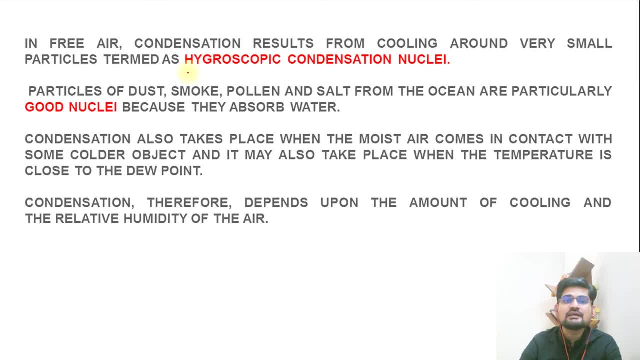 precipitation- that happens, or condensation that happens. so in free air, condensation results from cooling around a very small particle which is called hygroscopic condensation nuclei. remember we talked about the cloud formation and there we said that aerosols are important to actually give seat to these. remember, 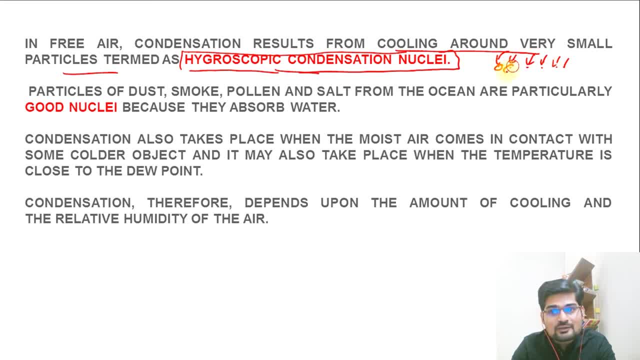 condensated liquid or ice crystals. so these are those nuclei is which provide base for this cloud formation. right, they are called hygroscopic condensation nuclei. so particles of dust, smoke, pollen, salt from the oceans are particularly good nuclei, as we say, for the absorption of this water. they give base to this. so 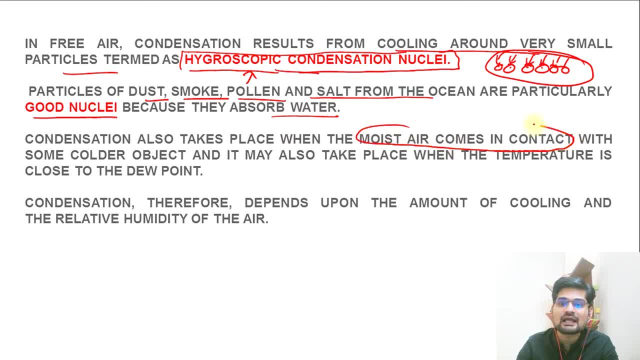 condensation also takes place when moist air comes in contact with the air in a with what Colder object? So remember this is also interesting. So it may also take place when the temperature is close to dew point. Now here is a catch: that if moist air comes, 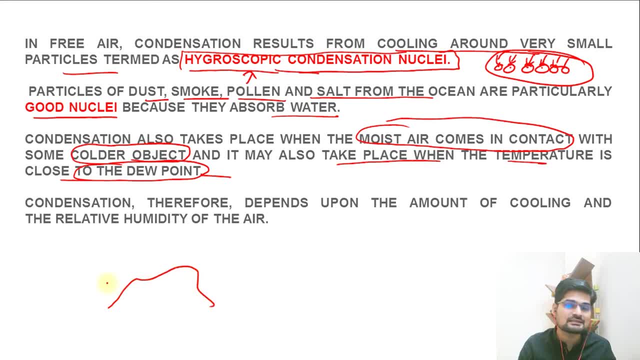 into the contact with colder object. it means if you are on the mountain slope and this is a moist air and here is a glacier, So what will start happening here? This will start condensating and it will start cloud formation here, or at least fog formation here, that we 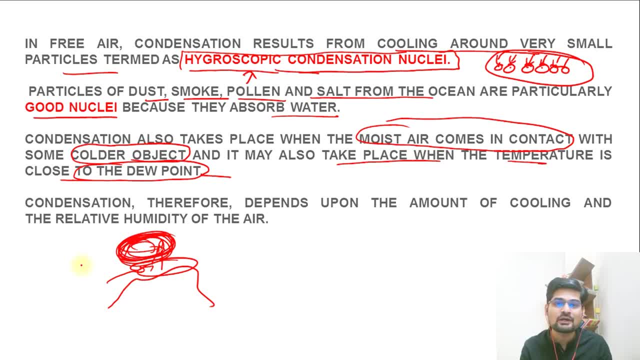 see. So whenever you go to the mountain areas and if you look into the hilltop during the daytime, when it is sunshine, what happens? Cloud starts forming, right That air is near this particular glacier or this particular mountain top, which starts cooling, So that 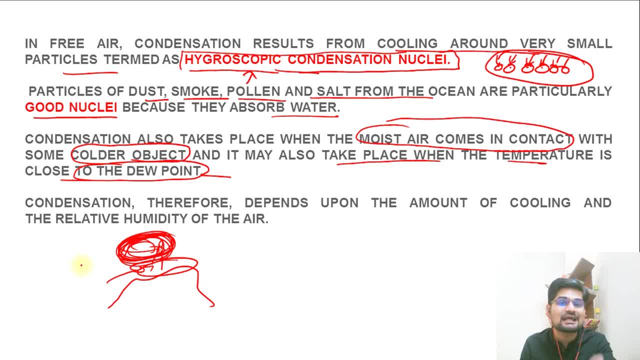 is why, after some time of the sunshine, you see lots of cloud rising on those particular areas of glacier right. So condensation therefore depends upon the amount of cooling and the relative humidity of air. This is what we need to keep in mind. So, amount of cooling, 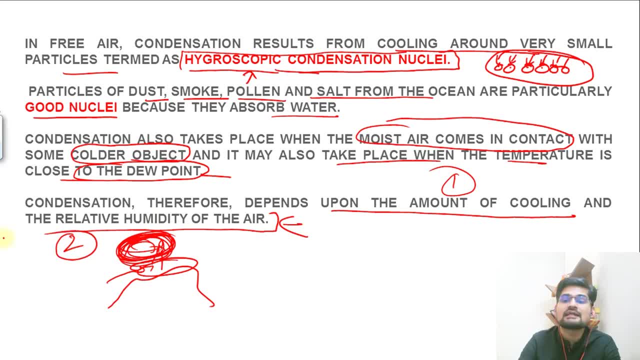 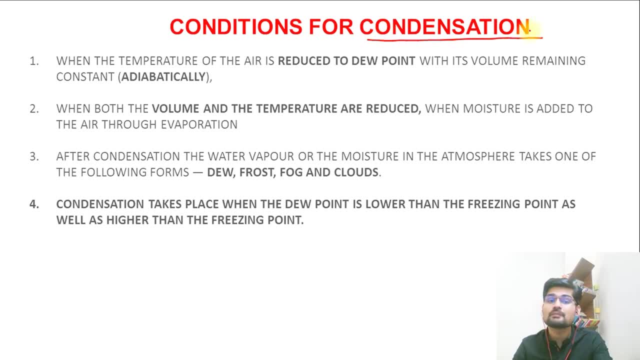 is the one factor and RH is the second factor That we need to consider. So now let's elaborate on the conditions for this condensation, which is important, which gives birth to various kinds of precipitation. So, when the temperature of air is reduced to dew point- Now, remember, when the temperature is reduced to dew point- 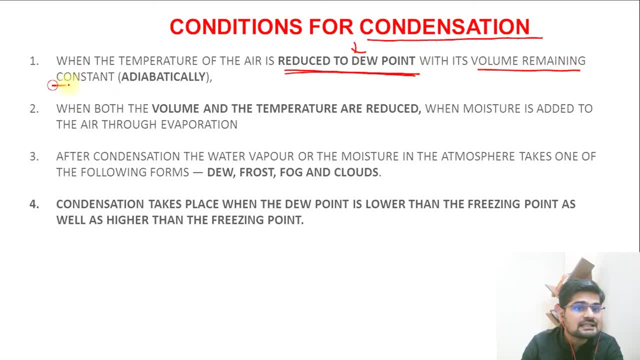 in this case what happens, Which is volume remaining constant. Now, remember, if volume is constant, then the process. remember what happens. It is adiabatic process, the PVT situation. So one is constant and there is variation in the other situation. So this: 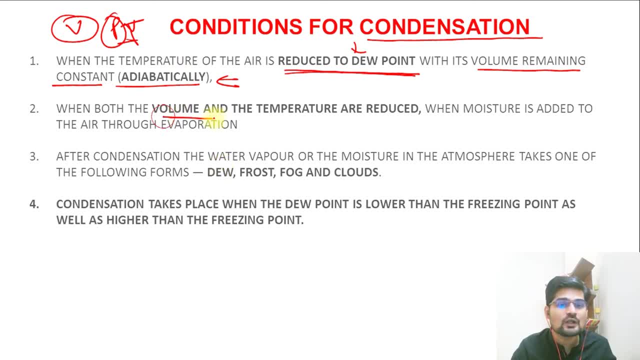 is what we say adiabatic process happens So when both the volume and temperature are reduced. Now remember if the volume and temperature, V and T, both are reduced. So what happens When moisture is added through the air? So when it happens When moisture is added to. 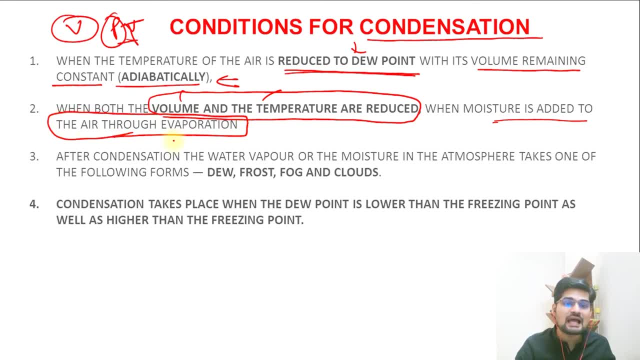 the air through evaporation. If moisture is added through this parcel of air through evaporation, what happens? It is getting more moisture. So here volume and temperature are reduced, but moisture is actually gaining. So there now see adiabatic changes happening. 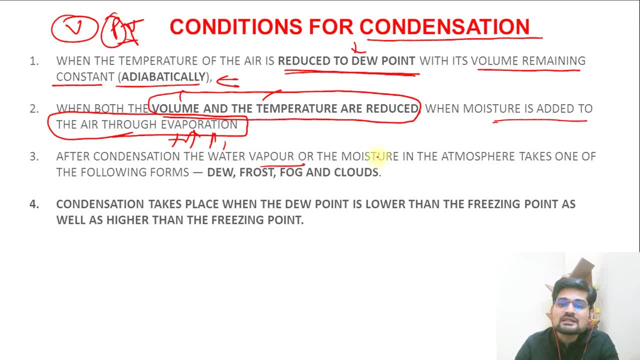 So, after condensation, what happens? The water vapor or the moisture in the atmosphere? Now, remember this point: water vapor, or the moisture that we say in the atmosphere, takes one of the following forms. which forms either it is dew, frost, fog and cloud formation. 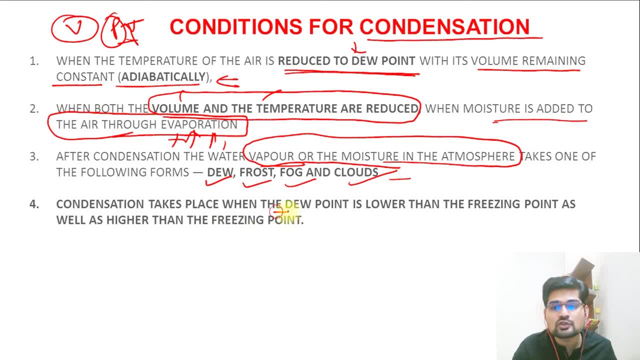 or rainfall happening. So condensation takes place when the dew point is lower than freezing point, in that situation as well, And if it is higher than freezing point as well. Now remember, if this is that line where I say, this is dew point, So even if it is higher, it will be a precipitation. Even if it is lower than value, it will be. 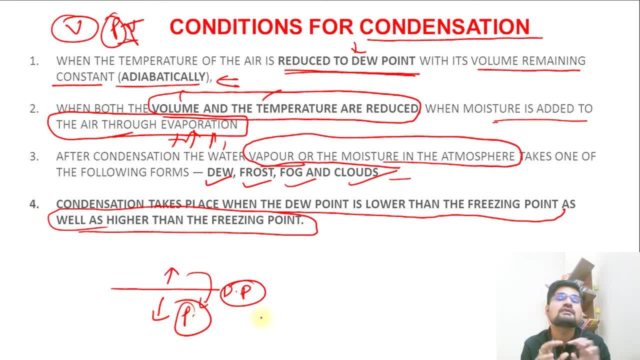 a precipitation. It's just that the precipitation will be of different kinds, right? So if it is below the dew point, it will be different. If it is above the dew point, it will be different. So now let's understand this further, more. So the forms of condensation will depend. 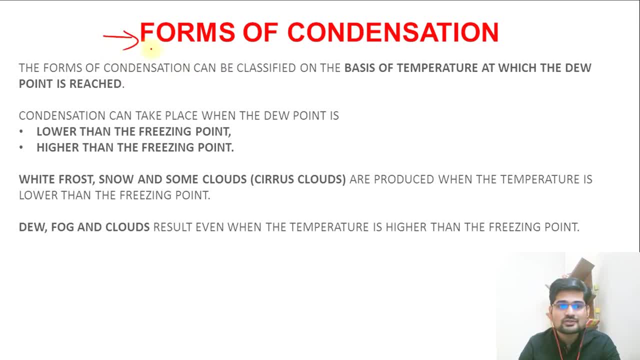 upon how. the temperature is there related to the dew point. So the forms of condensation can be classified on the basis of temperature at which dew point is Reached. So condensation can take place when the dew point is lower than freezing point and higher than freezing point, case one and case two. So when frost, snow and other clouds. 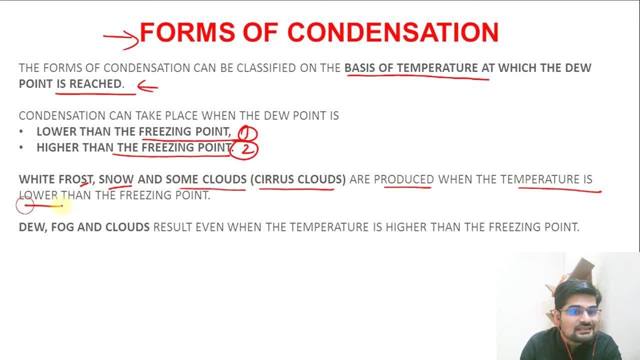 like Cyrus, clouds are produced when temperature is lower than freezing point. Now, remember, if temperature is lower than freezing point, then frost or snow and some clouds. Remember, if temperature is in negative, that is what? lower than freezing point, that is zero degree. 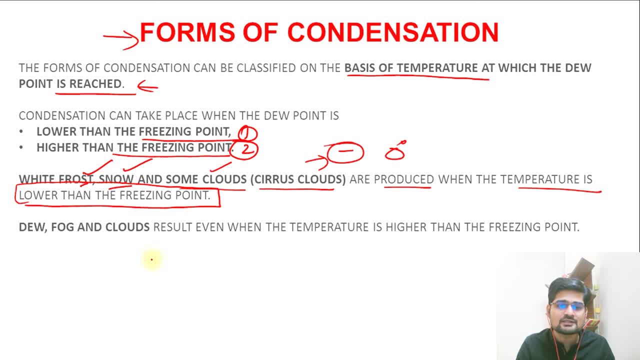 But if it is higher than freezing point, then it will be lower than freezing point, And if it is higher it is closer, but it is higher. It means it is one degree or 0.5 degree, So it is above the dew point, right. In that time what happens? dew is formed or fog is formed. 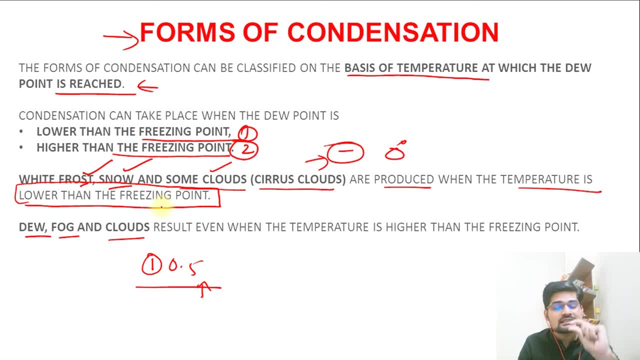 or clouds are resulted in that situation where it is a slightly above the dew point. So dew point is where the saturation happens. right, That is what we need to understand: that condensation also happens above the dew point temperature and below the dew point temperature, right. 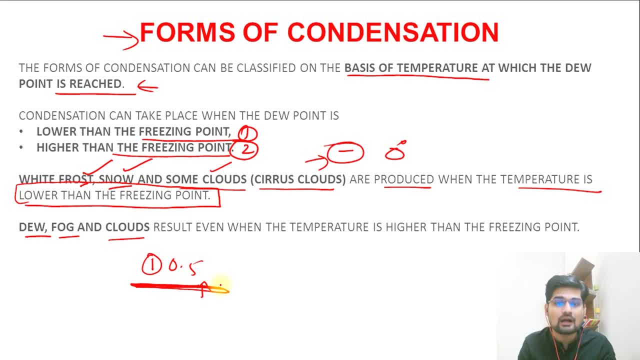 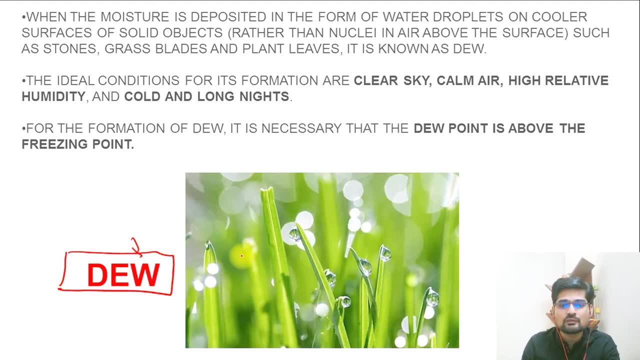 And in what ways the forms change. That is important to understand here. So now let's understand it one by one, the various types, So one. what we study clearly is called dew. If you remember what happens, this is grass where these water droplets are deposited. We say lots of dew is there on the ground. 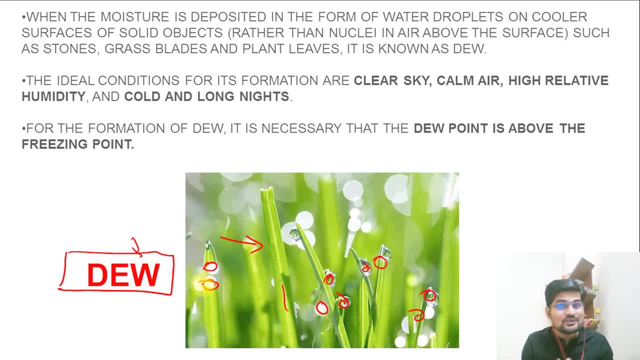 or moisture is there on the ground. Remember, in the cricket field, in cricket matches, dew condition. it has lots of role to play in terms of when you say there is a day night match, So when the moisture is deposited in the form of water droplets on cooler surfaces. 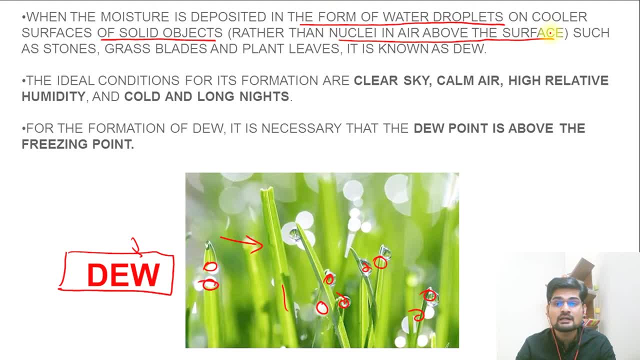 of solid objects. So these are the nuclei in air above the surface. Remember it is deposited on the other cooler surfaces such as stones, grass, blades, plant leaves. These are called dew because these are cooler surfaces. So if atmospheric condition and ground condition is a contrast, it means 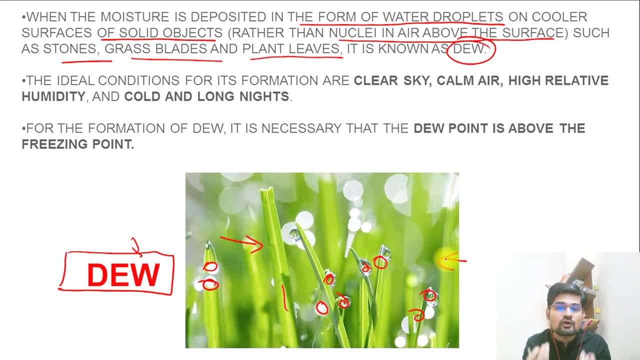 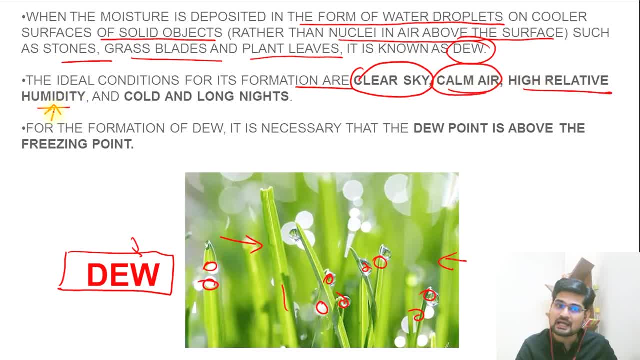 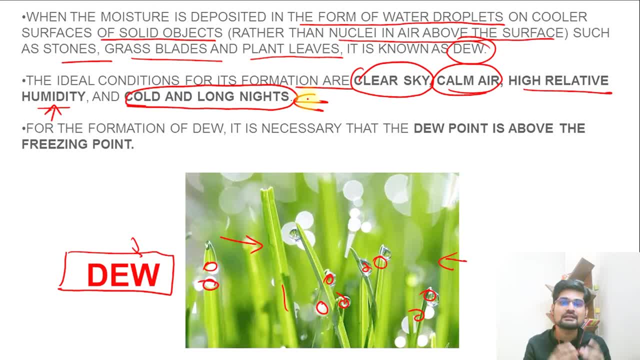 dew formation. So generally during the winters, when it is in the northern hemisphere, the advent of winters bring this idea of dew actually. So for the formation of dew it is necessary that dew point is above the freezing point. Now, if it is at the freezing point, remember. 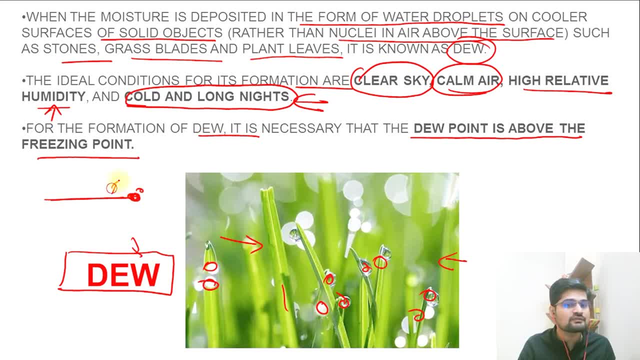 this is zero degree freezing point, then if it is not above the freezing point, it will not be in this dew format, in this liquid format. right, it will be frozen. so that is the reason. and next we understand is the frost condition. so remember, the frost is actually deposited in terms 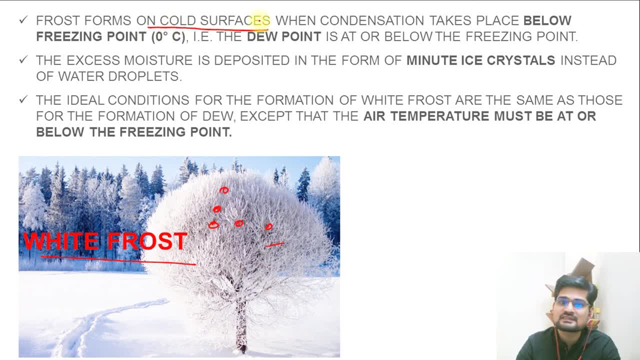 of the solidification. so frost forms on cold surfaces just like dew. but what happens here? the condensation here takes place below freezing point. so we see the difference here. dew was a water droplet and frost is actually hardened right, it solidified. that is important, because it is. 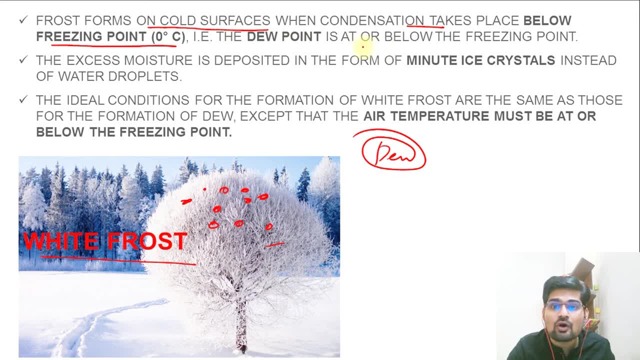 below the freezing point, that is, the dew point is at or below the freezing point. that is important. so dew point is below freezing point, it means it will be solidified. if dew point is above the freezing point, it means basically what it will be in liquid form. this is the basic idea, right? 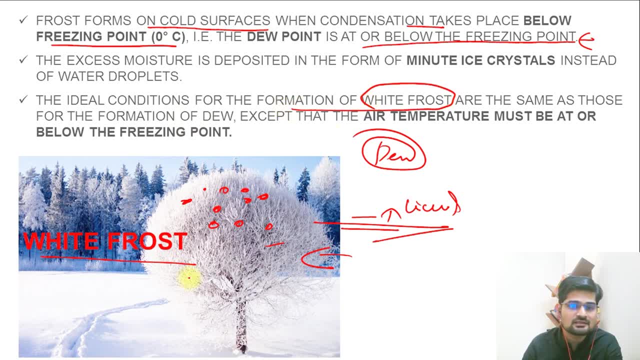 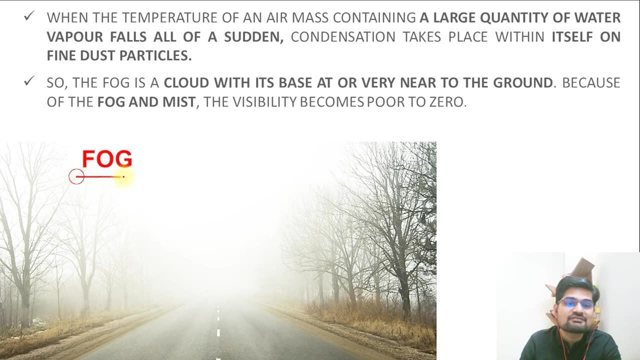 so the ideal conditions for the formation of white frost that we see here in this image also are same as those for the formation of dew, except air temperature must be at or below freezing point. that is when the frost formation happens. right now, the very famous that we see is the fog in. 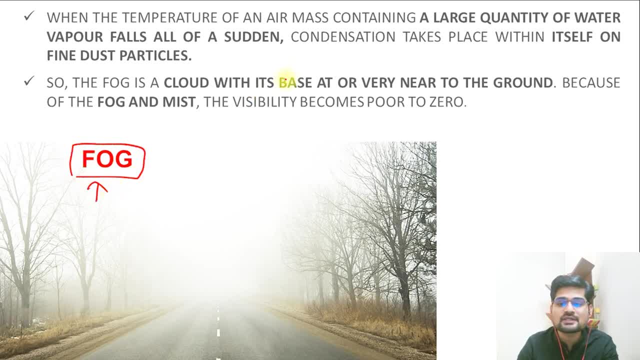 details. we are also going to learn separately on the fog. so when the temperature of an air mass containing a large quantity of water vapor falls all of a sudden, condensation takes place within itself on fine dust particles. now remember if dust particles are here, and this is a cool condition. 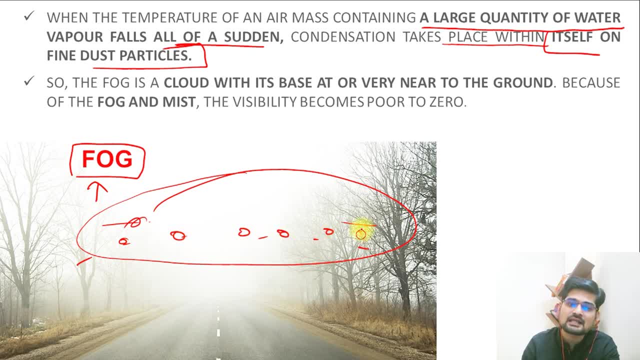 so what happens? condensation happens and these dust particles which are hanging in the air actually go into the air and get this particular moisture condensation right. so fog is a cloud only. but remember there is a difference: cloud is more denser, it is more bigger. in that way, if you see. 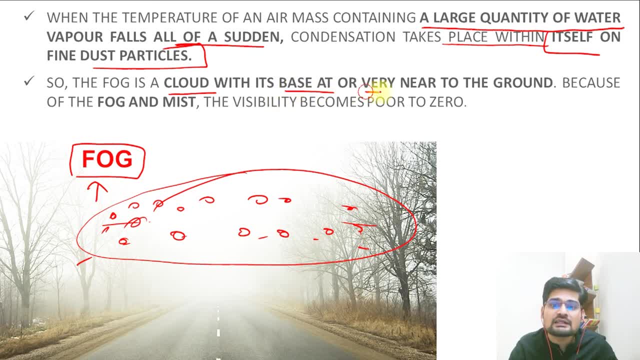 but it is kind of a cloud situation itself, with its base at or very near the ground. so remember, cloud formation happens at a certain level that is, one or two kilometers above the ground, but dew, but fog is actually like this. you remember, this is a road and this is where you see foggy. 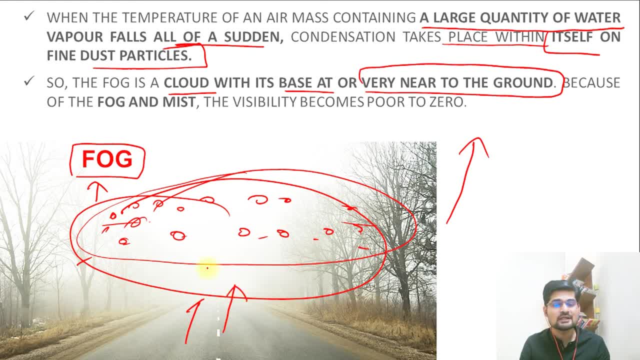 condition, even some meters, you cannot see further, so visibility becomes poor. so this is the difference, right. but the process of formation is very similar, like cloud, so it also requires condensation nuclei and which is closer to the ground. so if there is a dusty situation and it is a cold air in the ground surface, if it is, 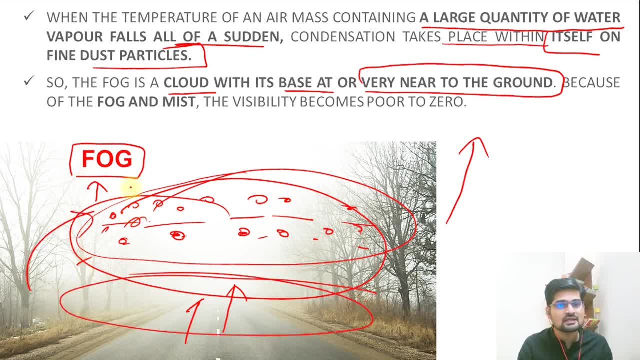 cold temperature. so moisture is there in the situation? if it is so, it will be a foggy situation, right? so this is what we see, that moisture is important, and specifically in the areas where you have lots of greenery, what you have, moisture is there through transpiration, right, so that. 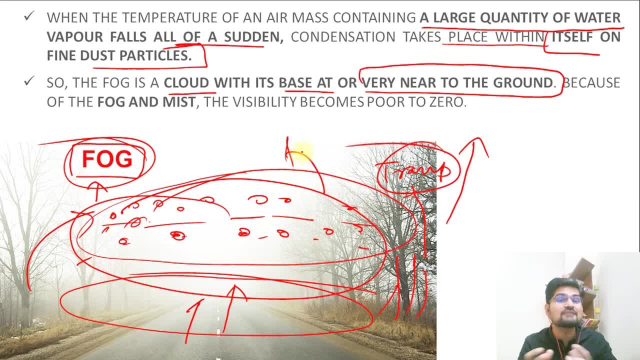 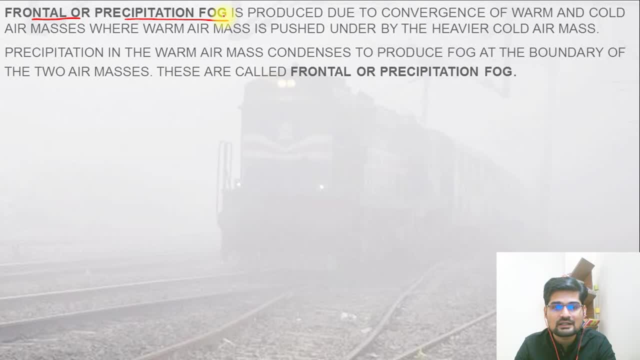 is already available. so that's where you have green areas with more fog in winter situation that you observe. now important is something called frontal or precipitation fog. that is also important to understand here. so it is produced due to the convergence of warm and cold air as well, where you have frontal formation. so warm air, cold air mixing. so there you have. 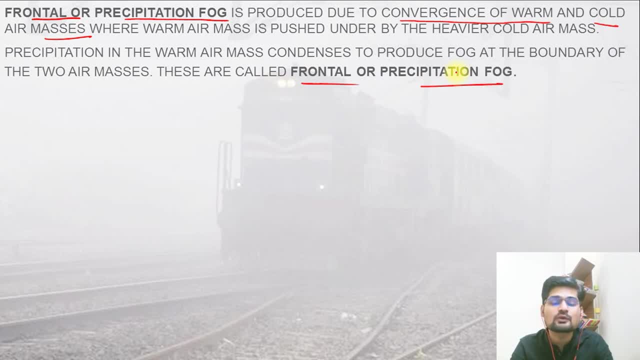 frontal or precipitation fog that develops. so, in details, we are going to learn about the fog in a separate lecture as well, for here, just remember, there is something called frontal fog, normally different from a convection fog, that is, rising air and then again cooling air. so this is. 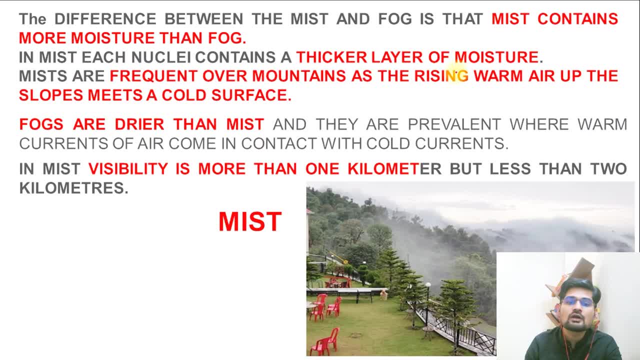 a frontal fog or precipitation fog that we also know. then we have something called mist. now, this is important to understand, that many people use mist and fog interchangeably. then what is the difference? the difference between the mist and fog is that mist contains more moisture than fog. 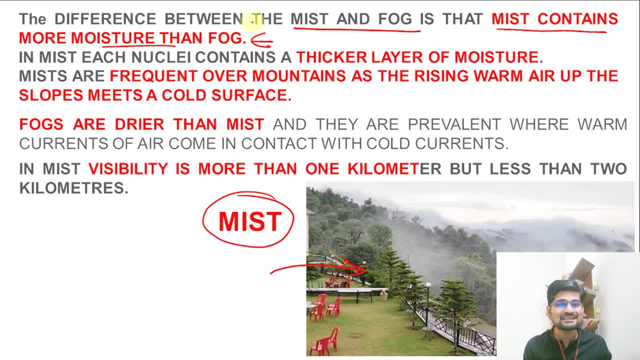 now. this is clear difference. so if you remember, if you say mist, it means it is more moisture content in the air. right, each nuclei contains a thicker layer of moisture. that is a significant difference, and mists are frequent over mountains as the rising warm air up slopes meet a cold surface. 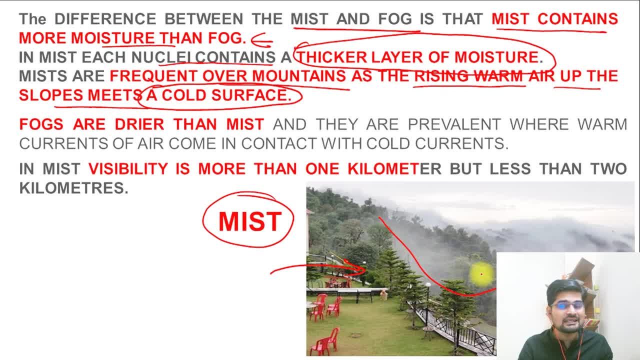 now remember, the inversion of temperature situation happens in the mountain and valley. that's where the misty situation occurs. so fogs are drier than mist. fogs have less moisture content. that's how we identify. fog is different from mist, but the conditions of formation are similar. so they are prevalent where warm currents of air. 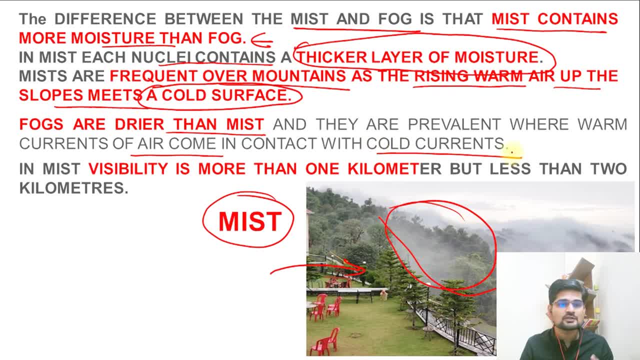 come in contact with the cold currents. that is where the fogs are formed. so in mist, visibility is more than one kilometer, but less than two kilometer. this is also a statistical data to remember that normally the range of visibility in the misty condition is not more than a kilometer. 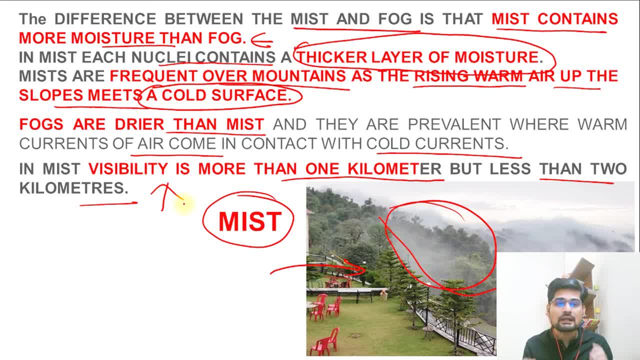 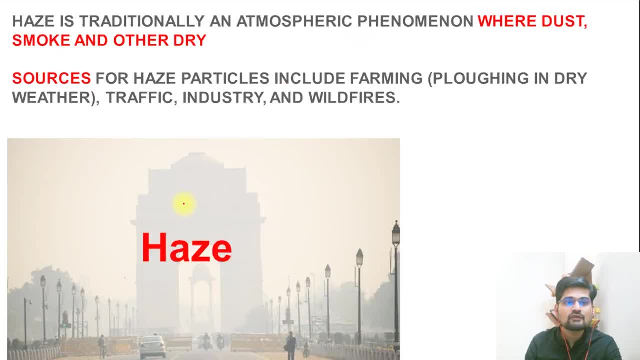 or two, so that is important. it also obstructs the visibility, but if you see the significant difference between a fog and mist- mist has more moisture content. that is important to understand- then what we have is something called haze. whenever we say it is hazy, what is it basically? haze is a traditional concept of atmospheric phenomena where dust 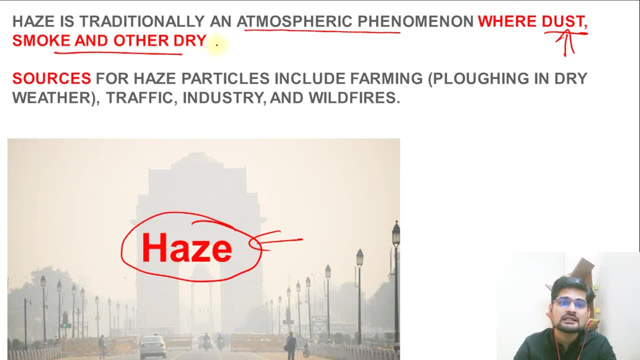 becomes important. so if it is too much dust or smoke or other dry air, what happens? it starts obstructing our or obscuring our visibility. so that is called hazy situation. and remember this haze has a thing to do with inversion of temperature, because if the temperature is 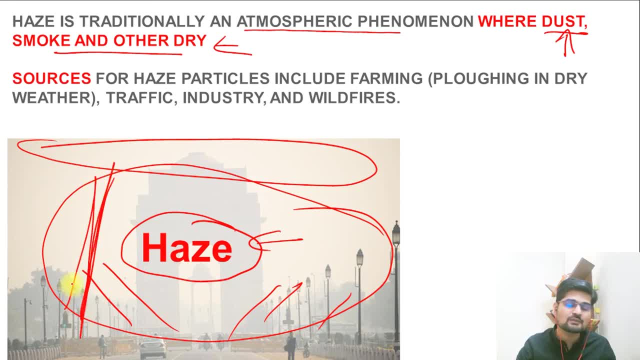 inverted. if inversion layer is here, this particular zone becomes hazy because of the addition of these pollution, like traffic industry wildfires. so this is a condition also that keeps happening where inversion of temperature is there, so it is also related to that, so it is called haze. now the last one. 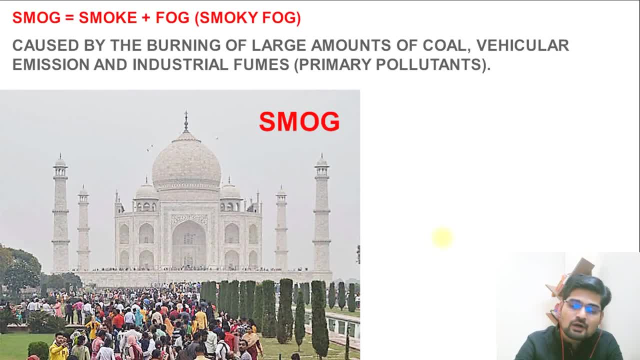 that we know is smog. and what is smog? smog is basically the combination of fog and smoke, so that is called smog. and if you look at this particular image of taj mahal, what do you see? the smoggy conditions because of the industrial pollution in agra. so it is caused by burning of.